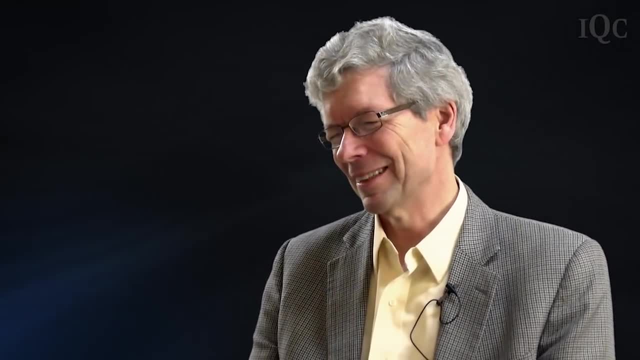 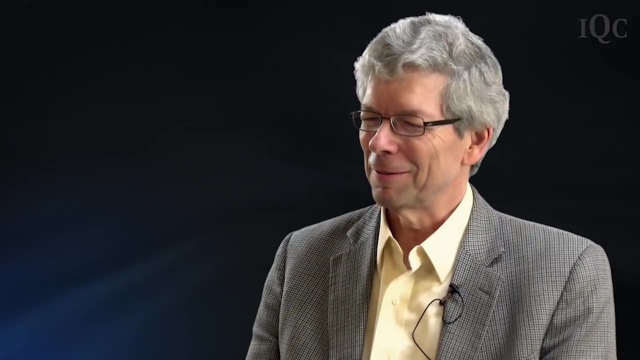 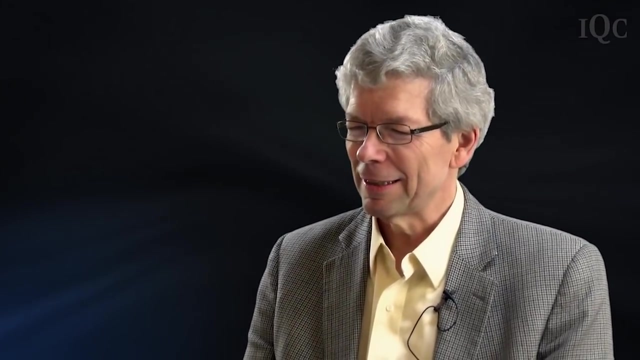 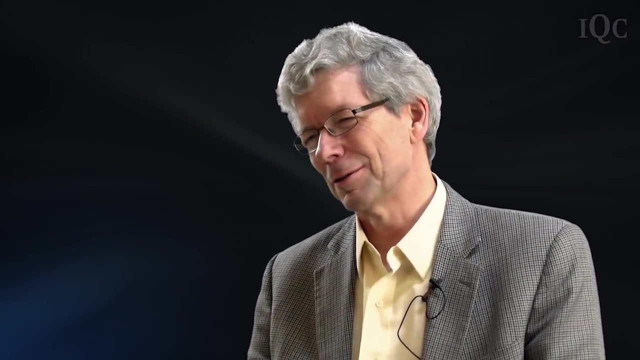 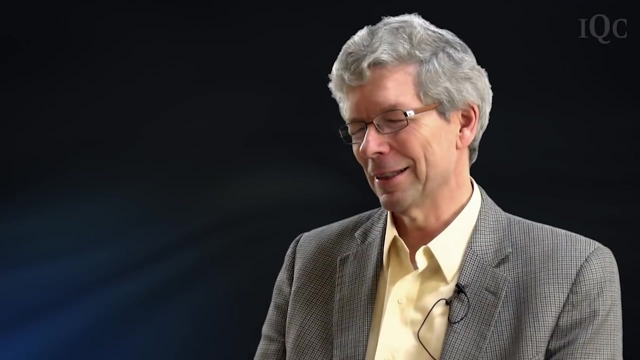 what used to be the distributor. It's now an electronic circuit that uses these Hall sensors and it has a number of other practical uses. The quantum Hall effect takes place in a very thin layer of electrons, essentially a two-dimensional sheet of electrons or electron gas, in a very strong perpendicular magnetic field. when the 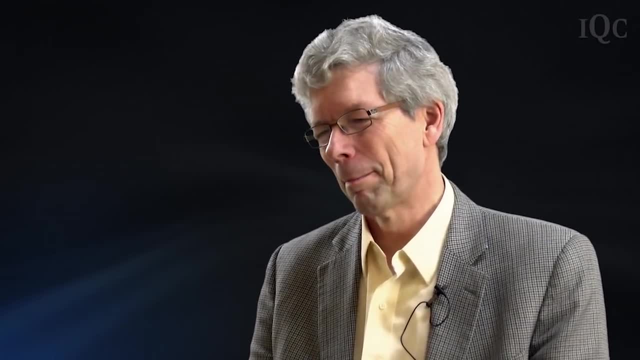 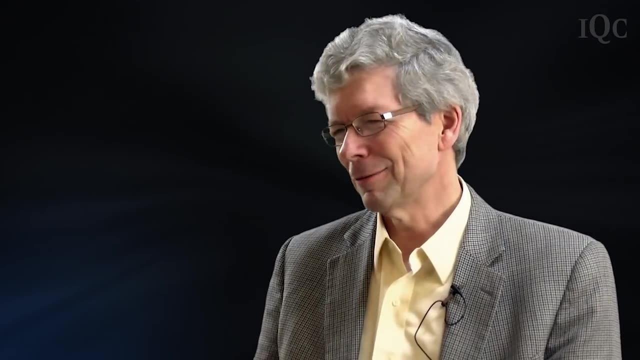 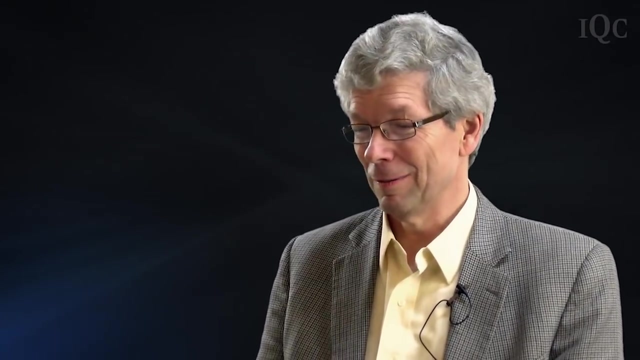 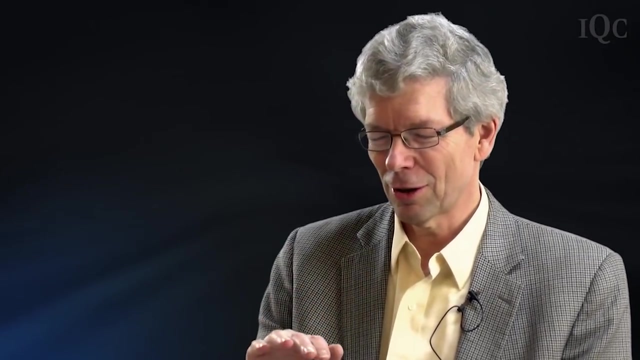 system is cooled down near absolute zero And it was discovered that, independent of all the microscopic details and the size and shape of the sample and exactly what the sample was made of and where any dirt and imperfections in the sample, nevertheless, when you've put a certain current through the sample, you've 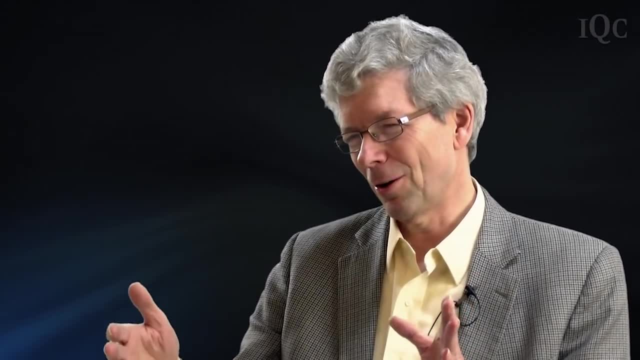 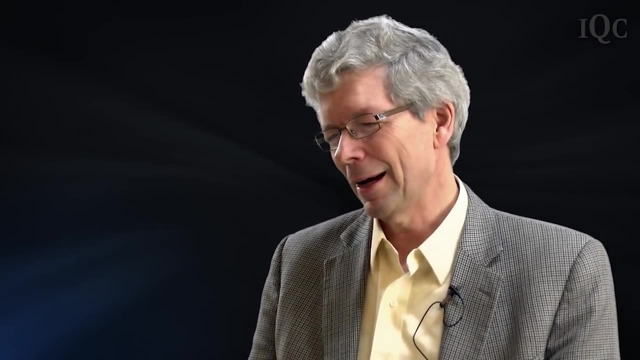 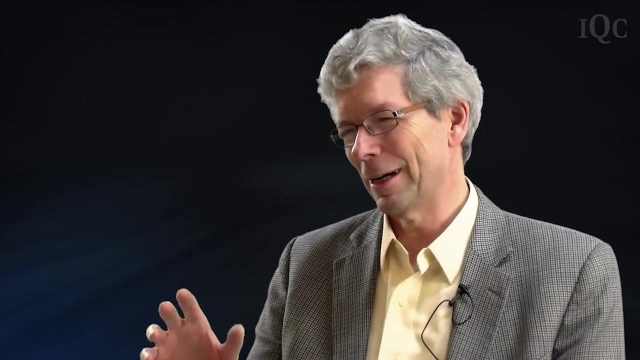 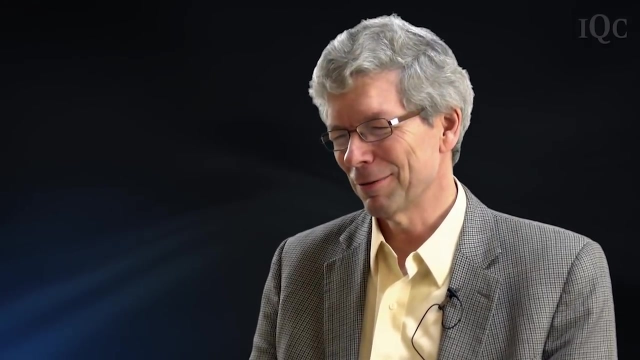 got a certain voltage And the ratio of that Hall voltage to the current has units of electrical resistance, Ohms, And it was discovered that you've got a universal value for that ratio And that resistance is called the quantized Hall resistance discovered by Klaus von Kutzing. 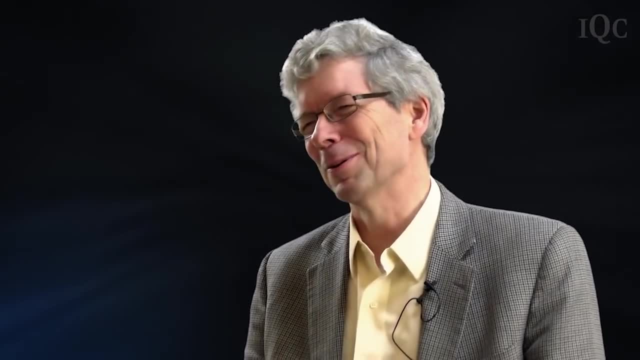 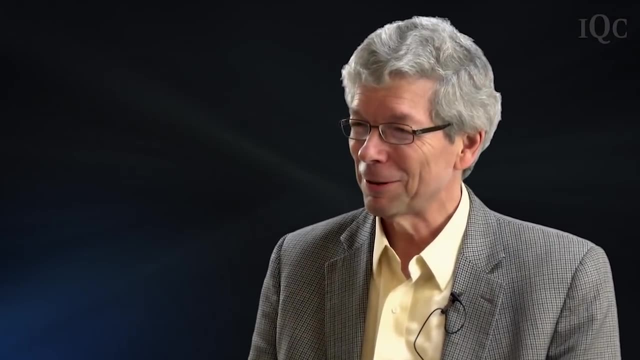 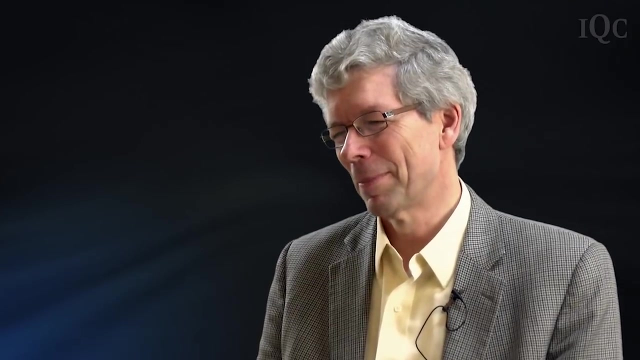 And it's 25,812.80 ohms approximately, And its value is actually given by the ratio of two fundamental constants: Ohms Planck's constant divided by the electron charge squared, Completely universal and fundamental. even though it's taking, this phenomenon is taking. 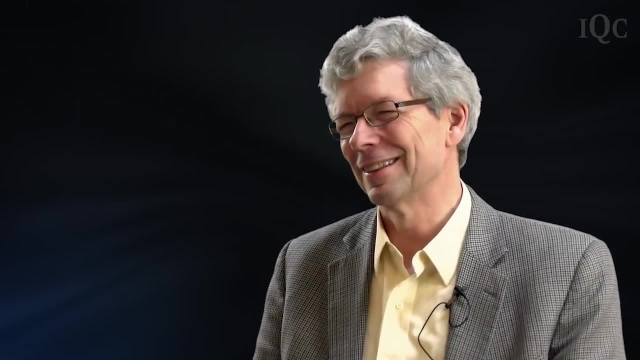 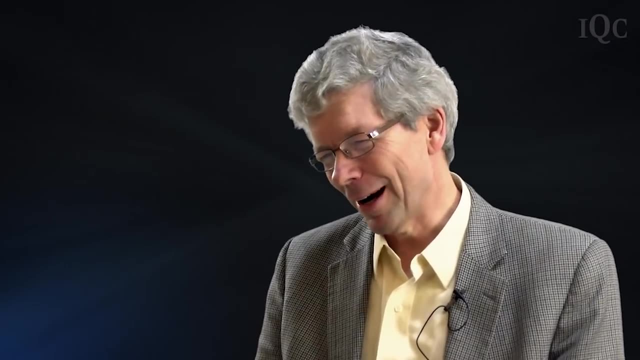 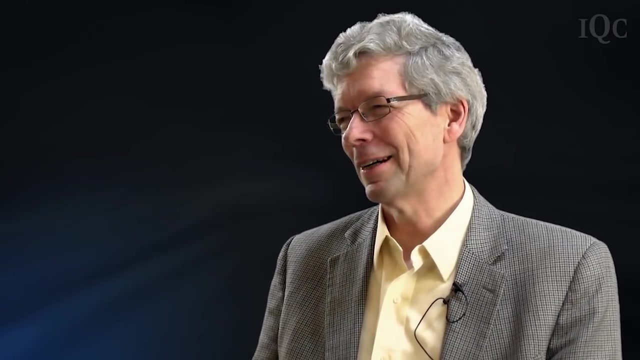 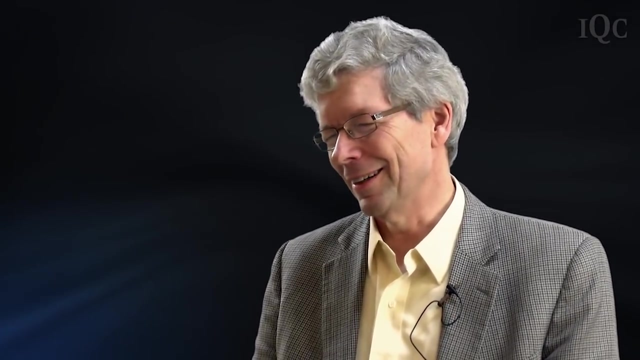 place in a dirty, not very perfect, hand-made, human-made sample. So that was a huge surprise. Then there was a second huge surprise: that some of the it's possible to see, you know, the fractional quantum numbers in this system and under other special circumstances, where 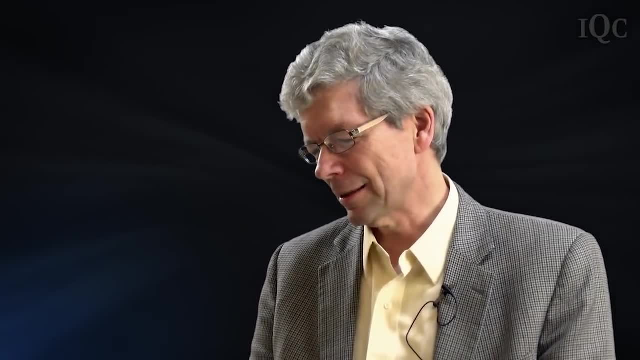 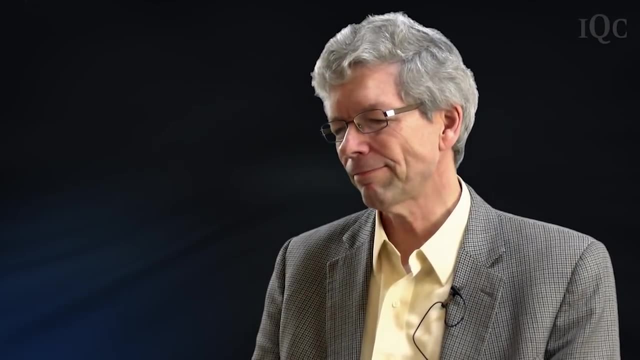 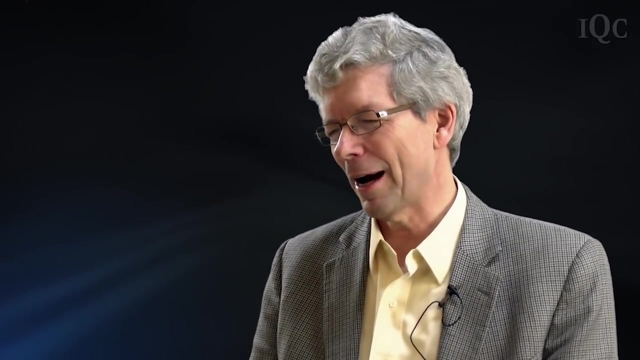 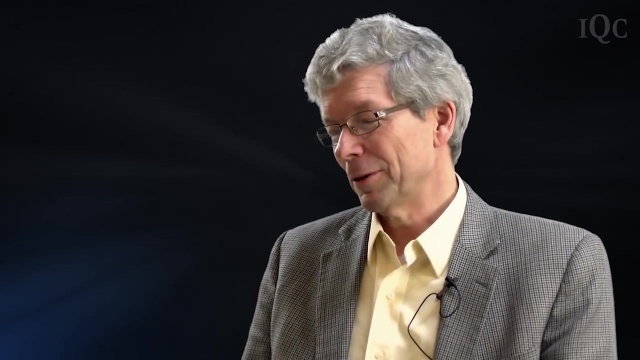 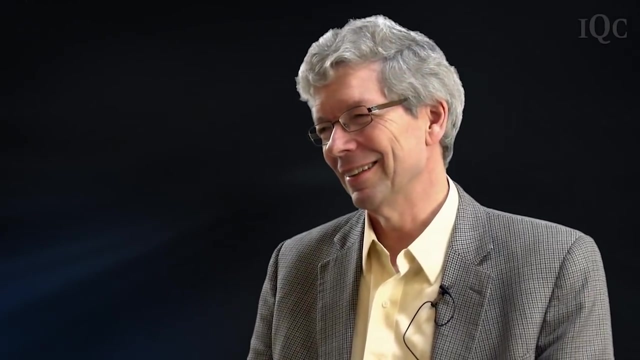 the electron interactions are important, So this led to a huge advance in our theoretical understanding of how a large system of interacting electrons can form a surprisingly subtle and complex quantum ground state. Further progress after that led to the realization that there could be even more complicated. 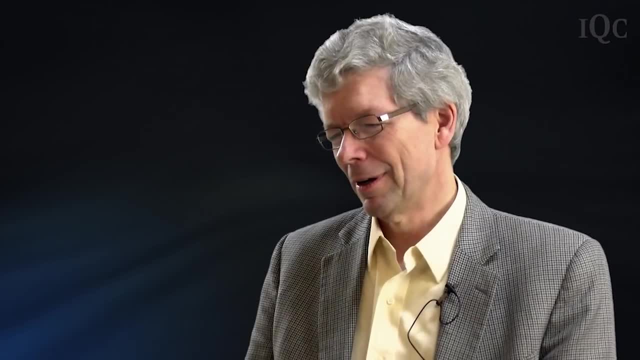 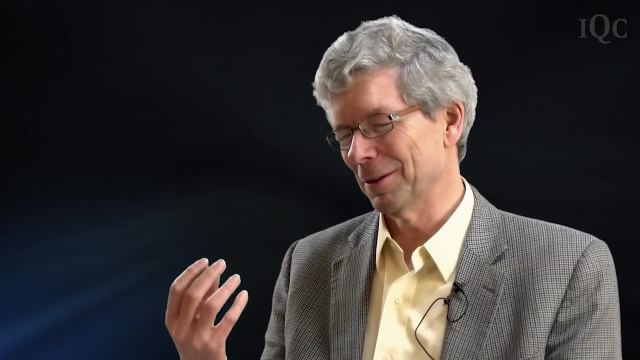 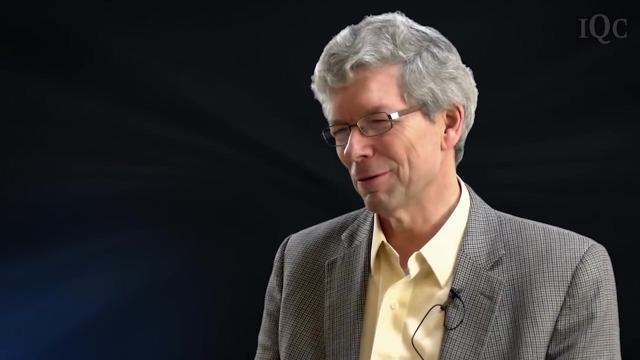 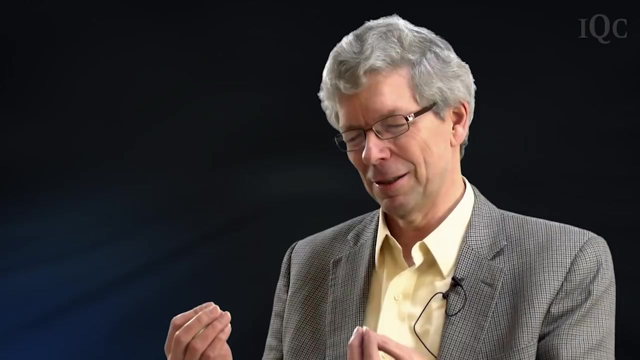 quantum states containing kind of quantum defects, quantum vortices, where there were little loops of current flowing around and people realized that those objects could actually be used to form quantum bits. And the way you would change the state of those quantum bits is to physically move them. 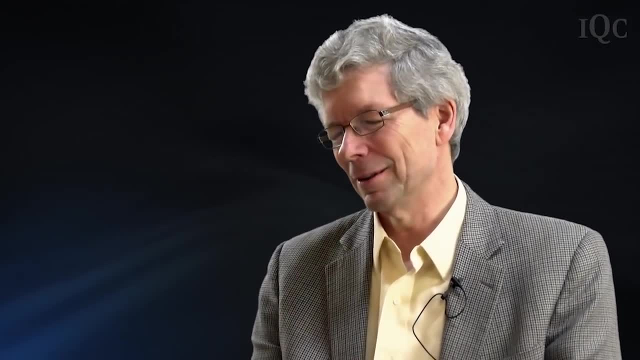 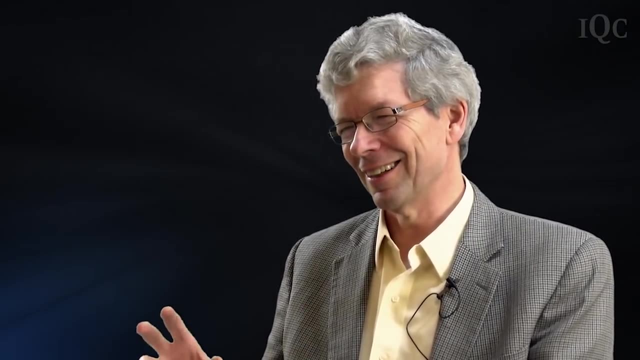 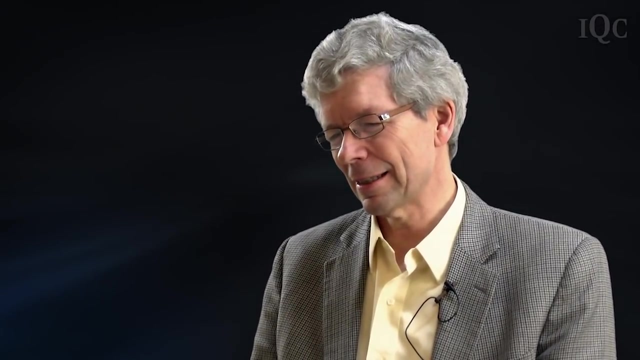 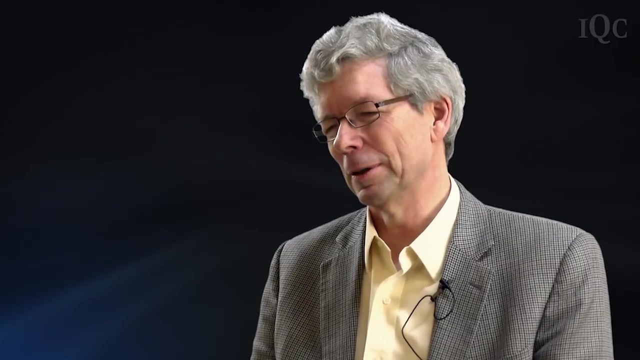 around each other, to braid them around each other, And the mere act of moving one particle around the other changes the state of this particle, And so there exists an idea for what's called a topology. It's called a topological quantum computer, in which the you would use these objects. 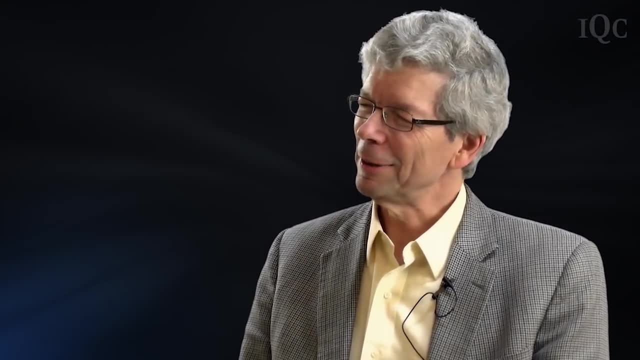 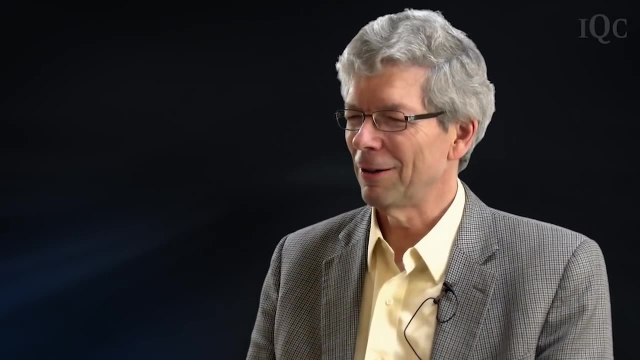 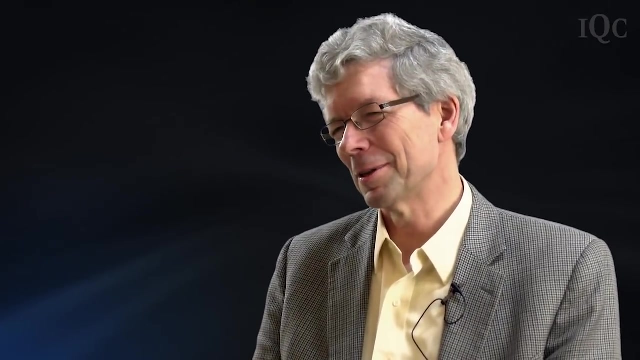 and braid them around to do the operations. The reason this is an interesting idea is I mentioned earlier that quantum systems are very sensitive to small perturbations and noise and imperfections, But this particular quantum state type of state is very robust against quantum. 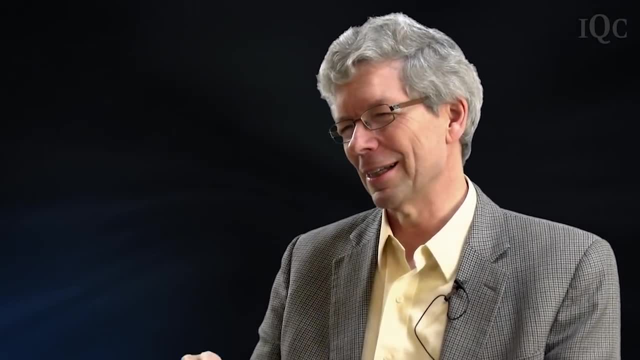 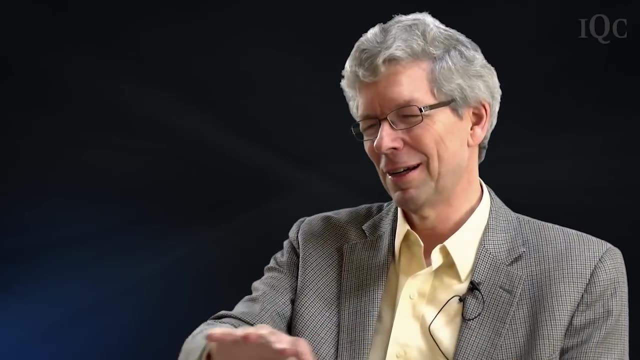 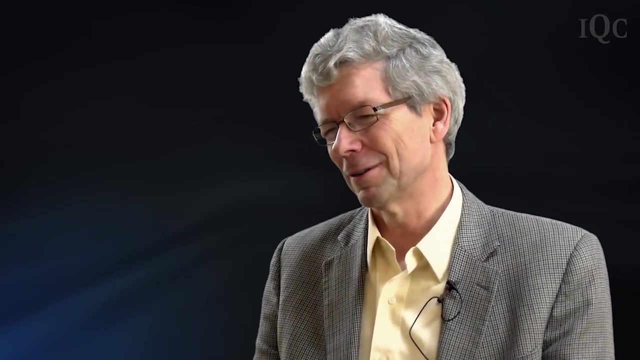 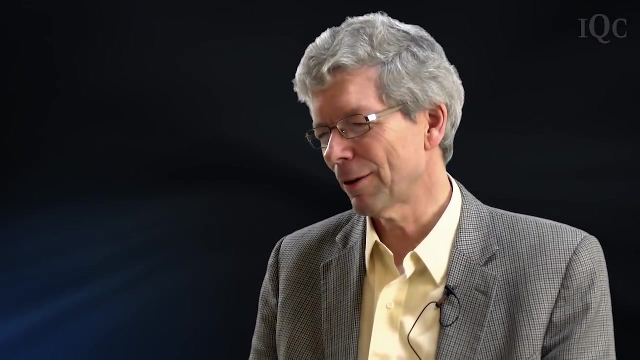 You can make local perturbations at any spot in the system and nothing happens to the quantum state, because the information is kind of spread out kind of holographically, it's spread out and shared amongst many of these particles And you can't no local perturbations can destroy that information. 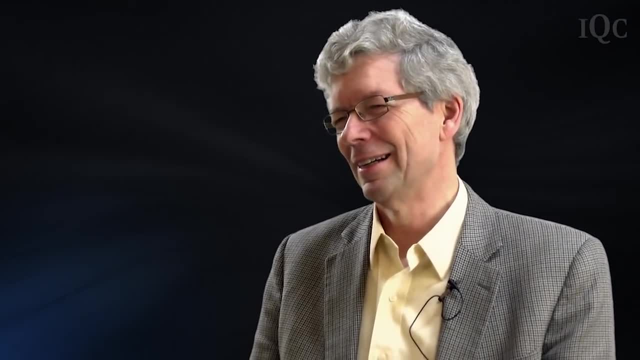 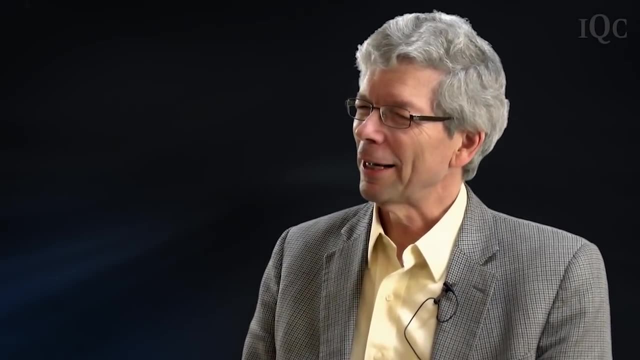 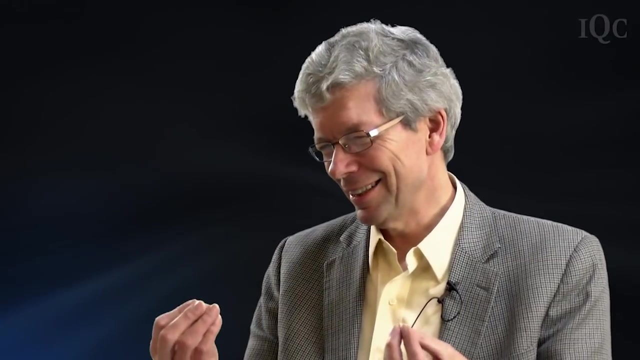 So the hope is that this would be very robust against noise and decay, And I think that's the key to this. Experimentally, it's very, very challenging And people are beginning. they definitely have seen these vortex objects. They have started to move them around each other. There's some evidence that you can see these fractional statistics and non-abelian statistics- the fancy words for these changes in state- When you Braid one around the other. But it's still very, very early days and the physics has not yet been really clearly. 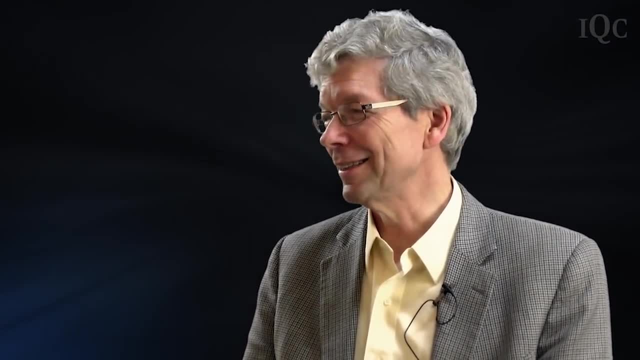 demonstrated experimentally, But again, it's too early to say it's not going to work for any piece of hardware.